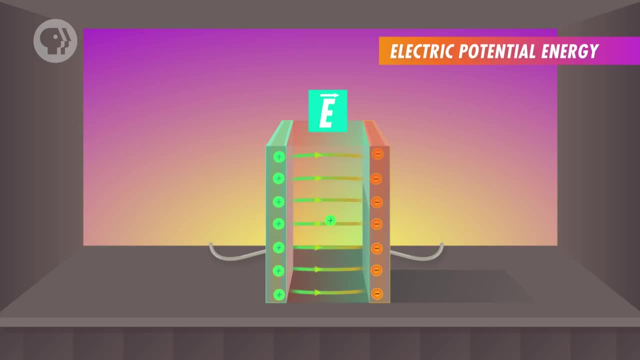 When we place the positive charge between the plates, the uniform electric field generates a constant force on it in the direction of the negative plate. If the test charge starts on the positive plate and travels in the direction of the electric force, we can calculate the work done on it by multiplying the electric force by the difference in the force. 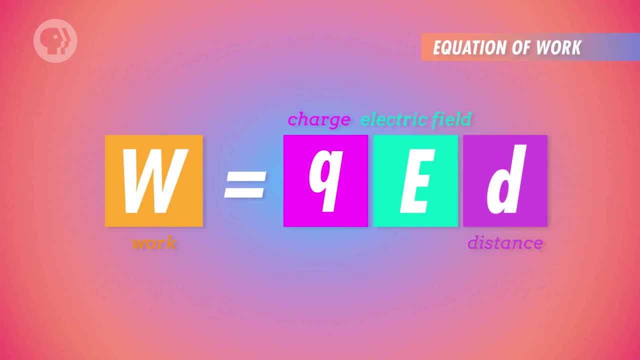 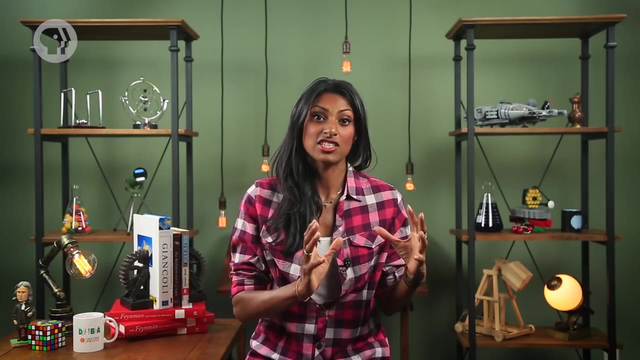 We also know that this force is equal to the value of the test charge times, the electric field. We can apply an equal and opposite force to the charged particle and move it across the capacitor as slowly as we like, so that the kinetic energy of the particle is negligible. 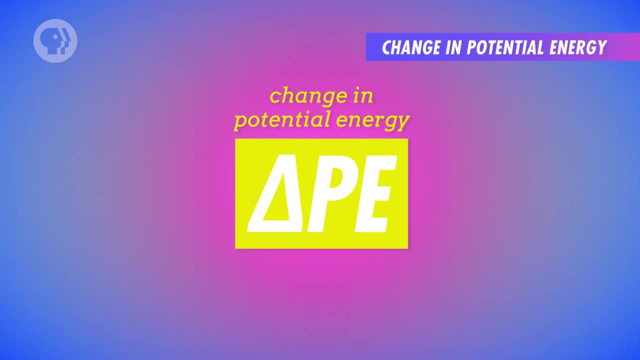 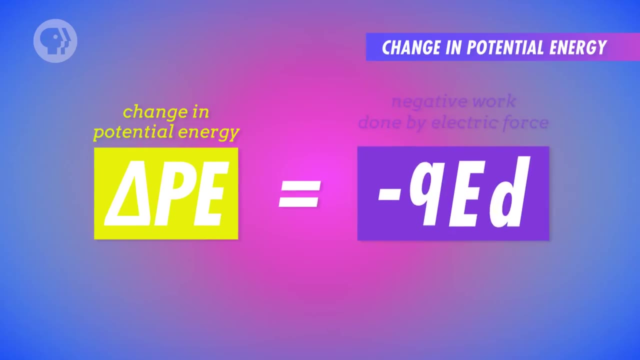 And because of what we know about the work-energy theorem and the law of conservation of energy, we know that a change of potential energy is equal to the work done by the external force or the negative work done by the electric force. So we've found the potential energy decrease of a single point charge in an electric field. 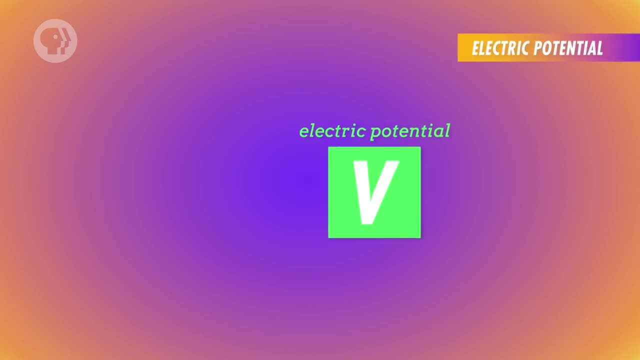 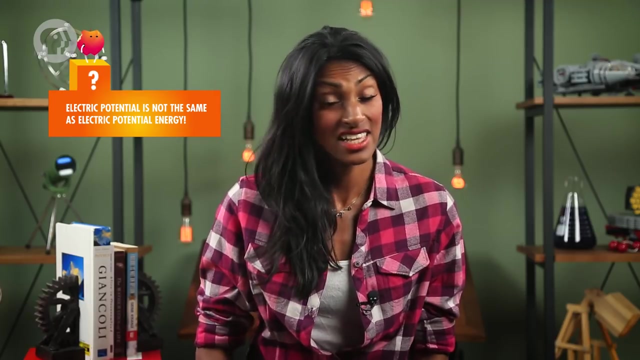 and this drop in potential energy divided by the test charge magnitude, gives us the electric potential energy difference per unit charge, also known as the electric potential. The electric potential depends on the electric field and the position, but it does not depend on the charge of the test charge. 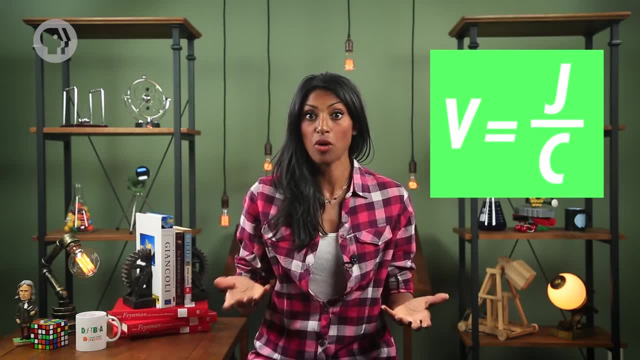 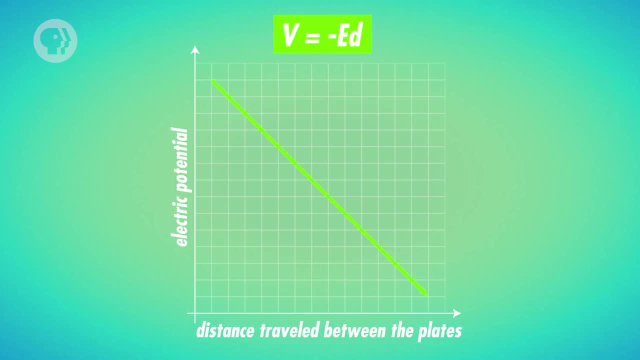 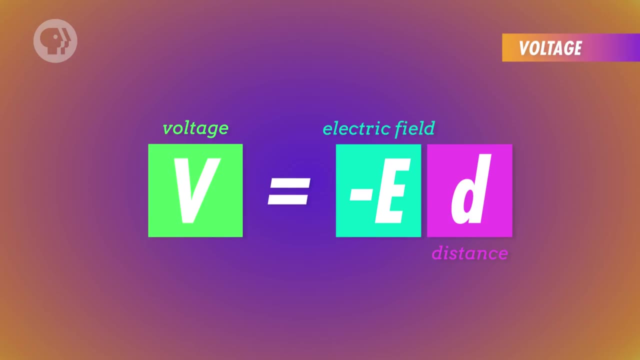 Now the units of electric potential are joules over coulombs, more commonly known as volts, And the electric potential difference is also called voltage, which is another way of describing a drop in electric potential. When we express it mathematically, voltage is equal to the negative electric field times the distance between the capacitor plates. 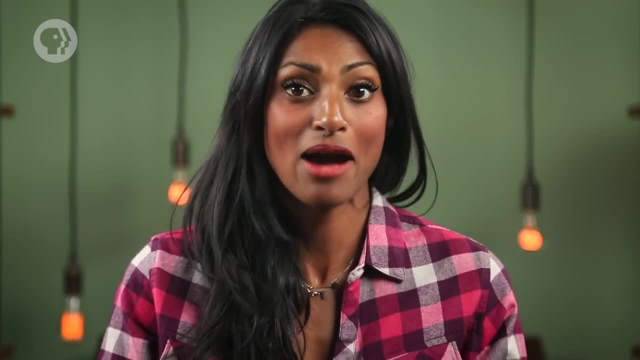 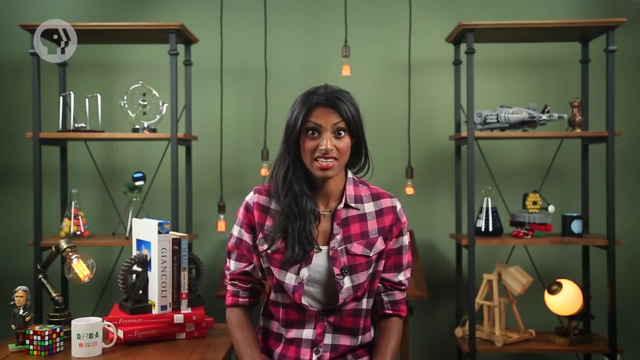 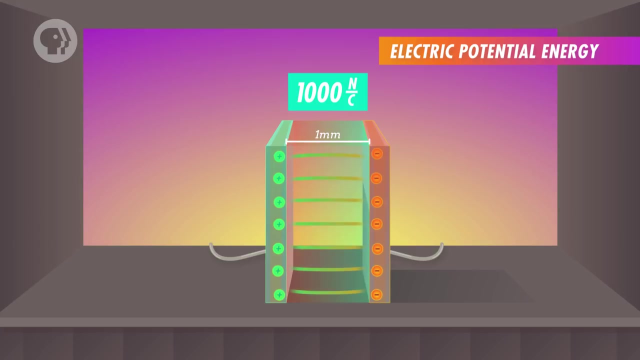 OK, we've used our hypothetical positive test charge to describe how much voltage is present across the charged capacitor. Now let's put our new expressions to the test and find the electric potential difference in a real scenario. Let's say we have a capacitor with plates 1 mm apart and an electric field of 1000 N per coulomb, which is the same as 1000 V per meter. 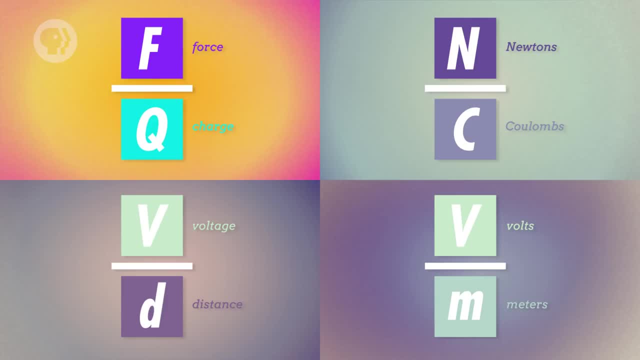 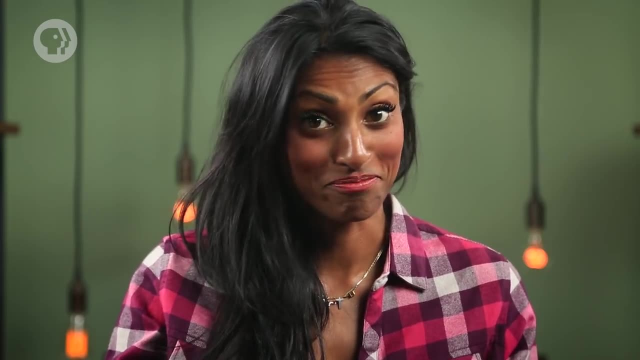 The electric field can be found by dividing force by charge, Or, for that matter, newtons over coulombs, as well as voltage over distance or volts per meter. They all represent the same values. So say, we multiply 1000 V per meter by 1 mm, we find that the capacitor has a voltage of 1 volt. 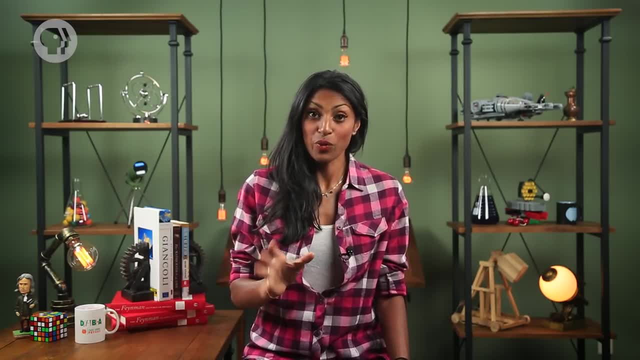 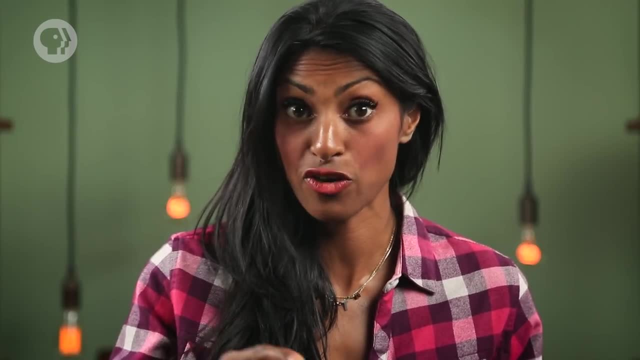 Now, since a capacitor creates a uniform electric field, we can assume the electric force is constant and that it acts in the direction in which the test charge moves, And as it moves the potential will decrease more and more. We can represent this voltage drop visually. 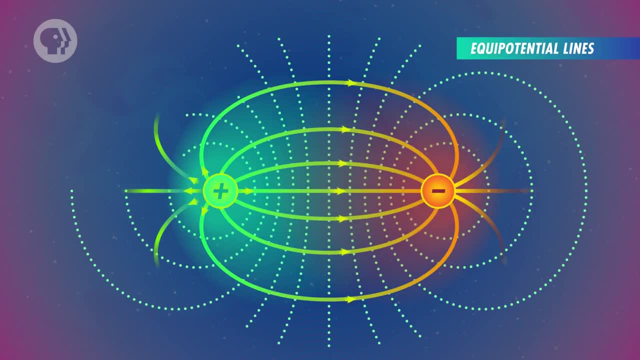 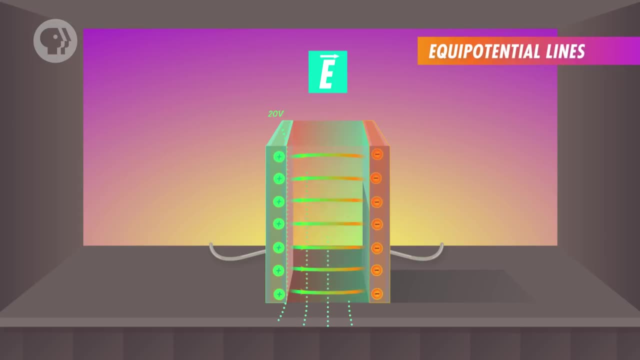 By drawing lines along the locations where all the test charges have the same voltage. These are known as equipotential lines. In a capacitor, these lines run parallel to the plates, And each line that's closer to the negative plate has a lower electric potential or a lower voltage. 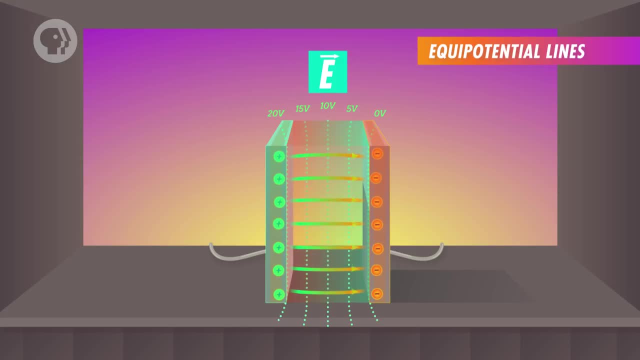 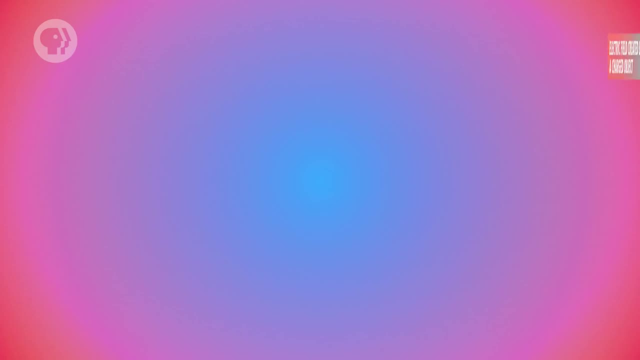 And these equipotential lines are always perpendicular to the electric field. So far, we've learned how to calculate electric potential for capacitors, But can we apply the same ideas to point charges? Well, we know the equation for the electric field generated by a point charge. 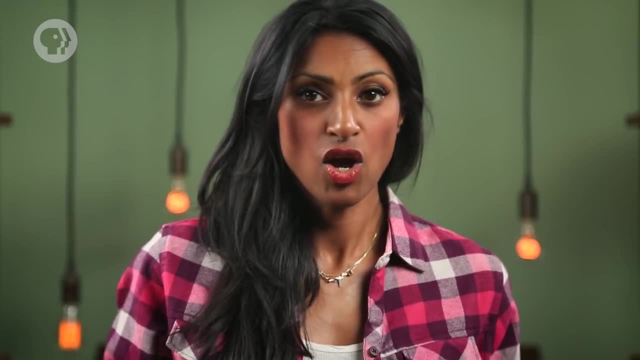 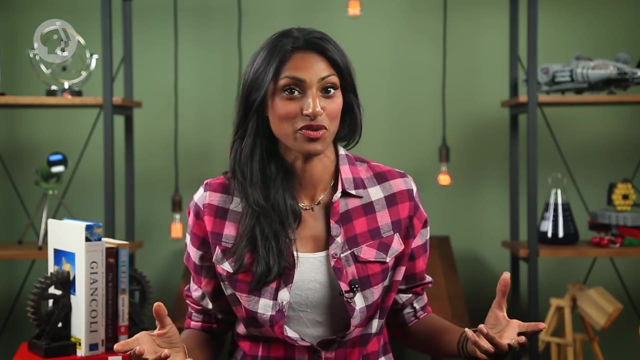 But since there's no uniform field like there would be with a capacitor, we can't use all the equations that we've been using so far. Finding the electric potential created by a point charge is like finding the difference in potential energy per unit charge between the spot right next to the point charge and somewhere infinitely far away. 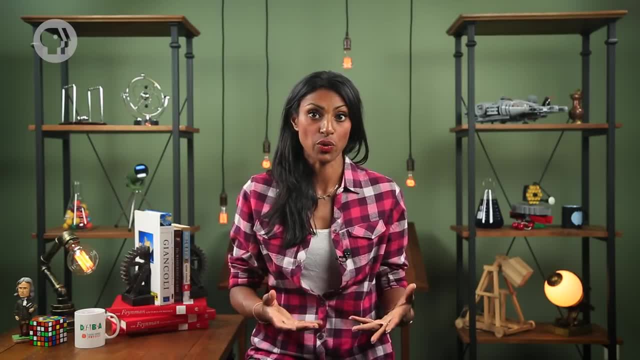 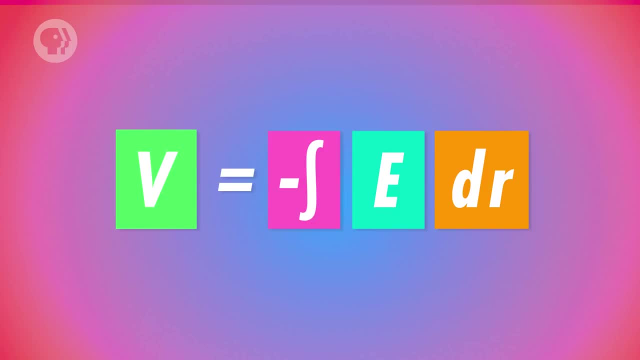 If a small charge object with the same sign was next to our point, charge Q, it would start with a high electric potential while it was close by and have a very low electric potential as it got farther away. So we can calculate the total electric potential possible by integrating the negative electric field from infinity to zero. 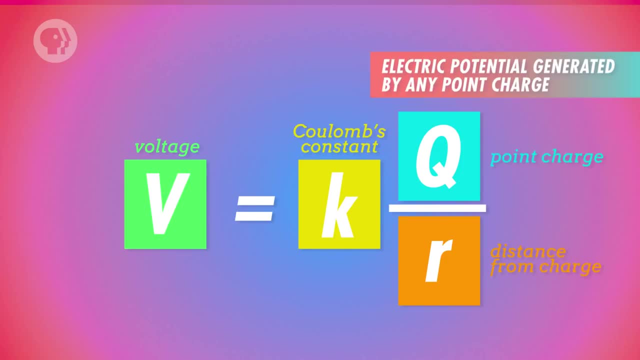 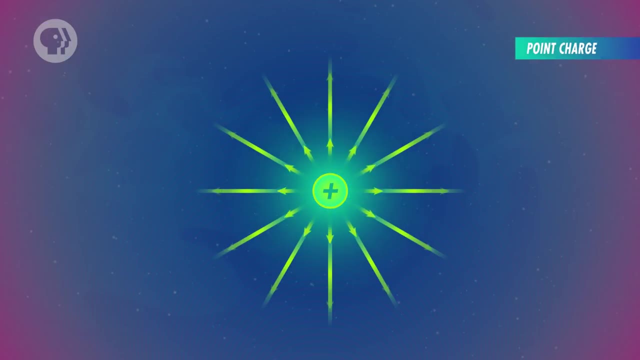 We're left with an equation that describes the electric potential generated by any point charge, And we can map equipotential lines for point charges in the same way we did for the capacitor. For a point charge, the equipotential lines look like circles of increasing size around the charged particle. 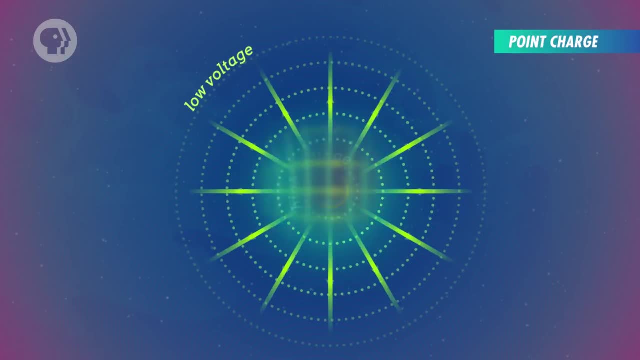 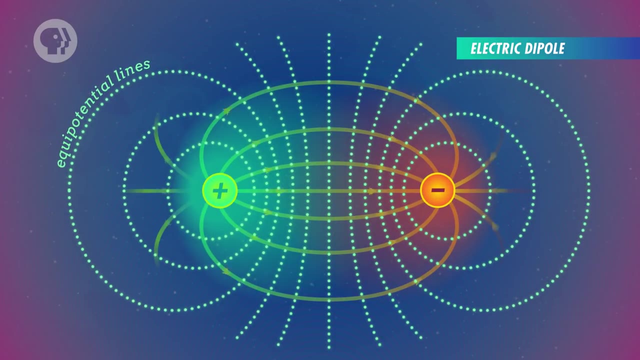 The farther away from the point charge, the lower the voltage. And for an electric dipole which is one positive point charge and one negative point charge, the electric potentials from individual charges can be added together. Here you'll see that each equipotential line is not a constant distance from a point charge. 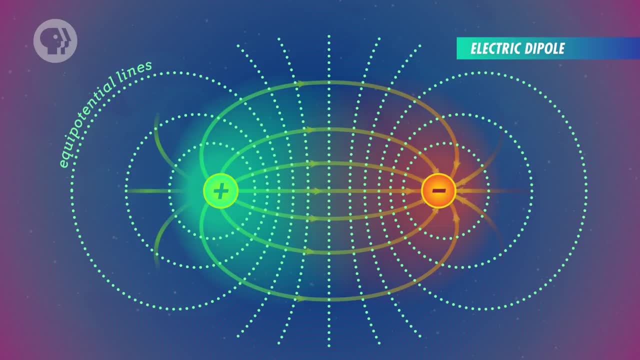 That's because you've got two point charges with their own electric fields. so a test charge on the right side of the positive point charge won't have the same potential as one the same distance away on the opposite side. Now let's go back to potential energy in capacitors, because it's largely why capacitors are so incredibly useful. 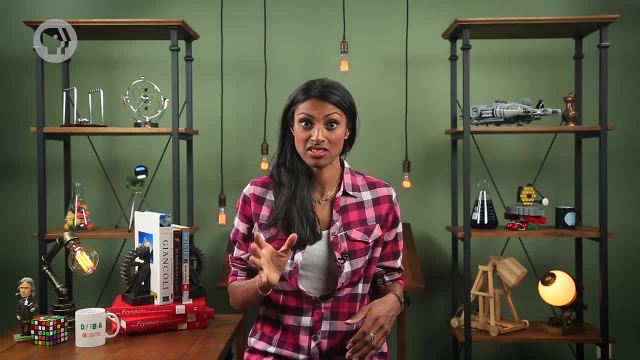 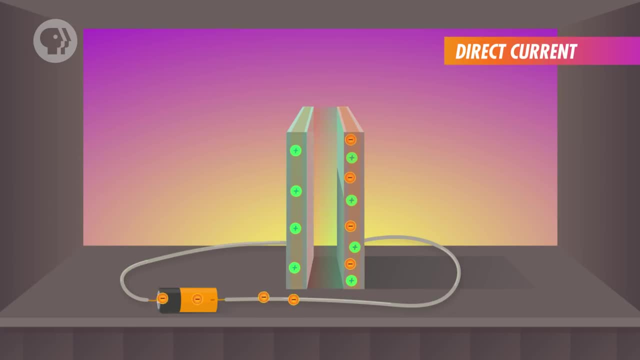 From defibrillators to electronic components. when a capacitor's plates store electric charge, they're actually storing energy. If you connect a battery to a basic circuit that contains only a capacitor, the battery causes charge to move from one plate to the other through a capacitor. 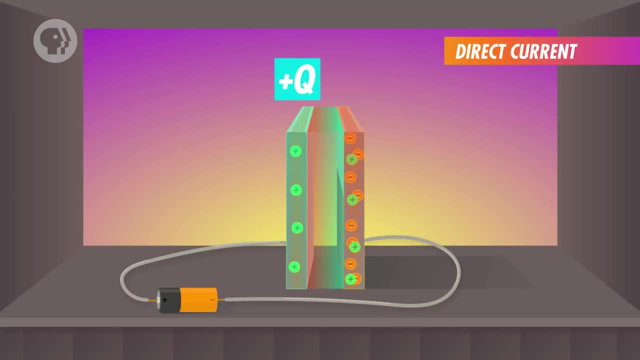 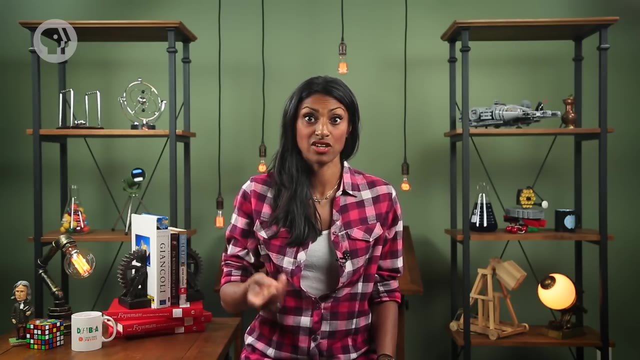 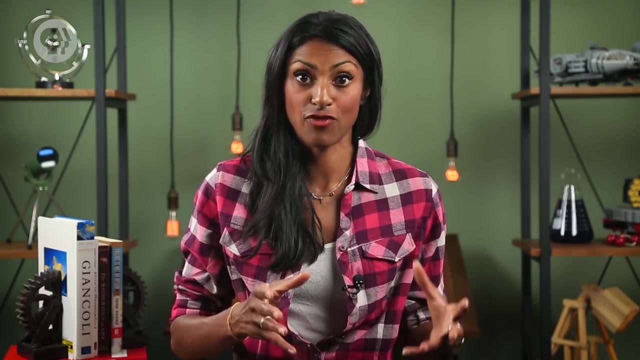 This results in one positively charged plate and one negatively charged plate, But the capacitor hasn't gained any net charge. There's just as much positive charge on the positive plate as there is negative charge on the negative one. So the battery uses its only electric potential to generate a current that transfers voltage in the battery to voltage in the capacitor, giving the capacitor a certain amount of potential energy. 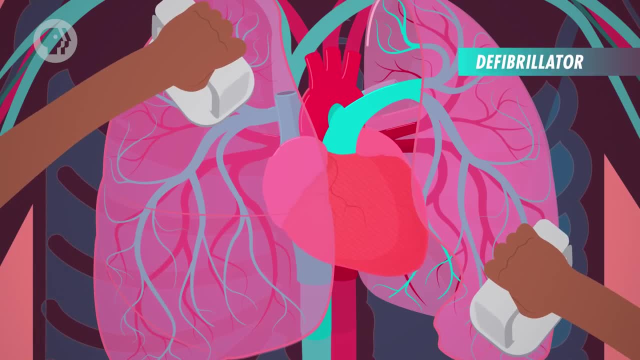 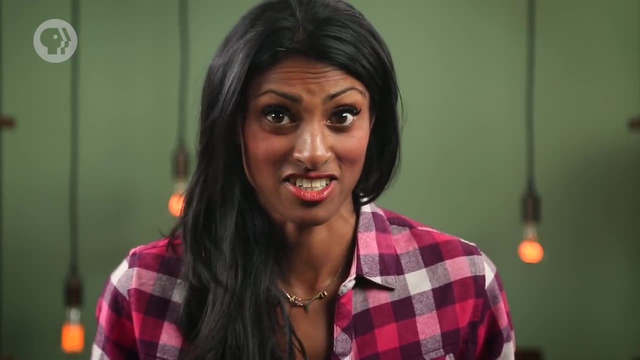 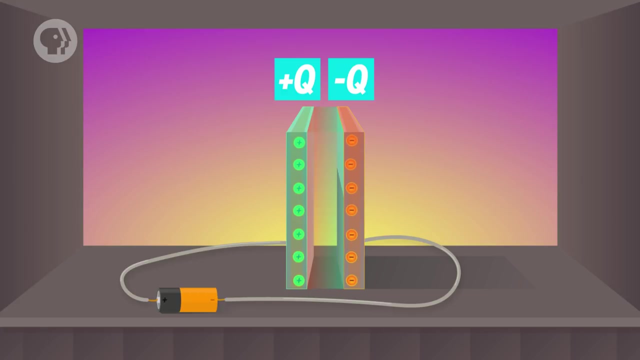 For our defibrillator. this energy is quickly turned from potential energy into a jolt of electricity through the human body. Now if you're trying to save a life, you want to make sure you're getting just the right amount of energy. So to measure how much charge a capacitor can store, we can use a battery in our circuit to create a voltage between the plates and then divide the charge in each plate by that voltage. 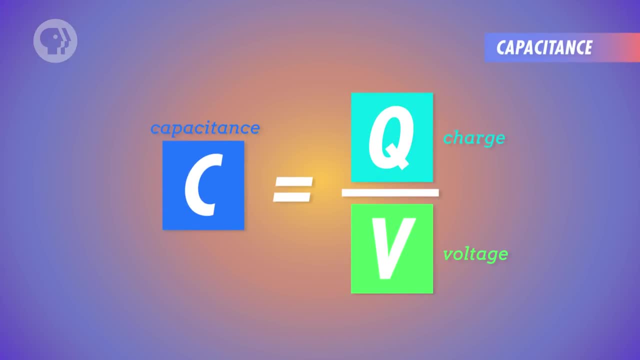 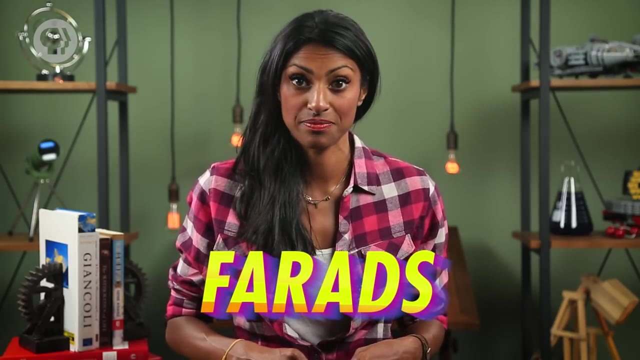 This value is known as capacitance: how much charge a capacitor is able to hold. Capacitance uses units of farads, with one farad equal to one coulomb per volt. Typically, capacitance values are very small, so we often talk about capacitors in terms of microfarads or nanofarads. 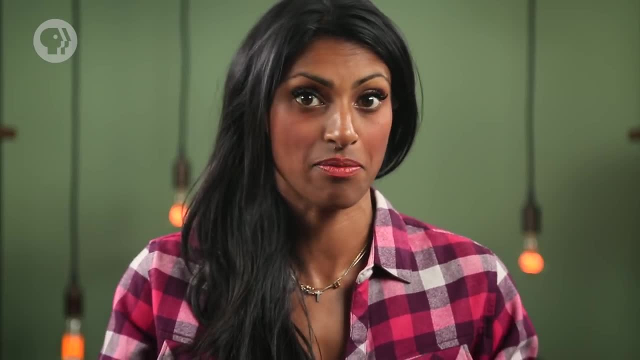 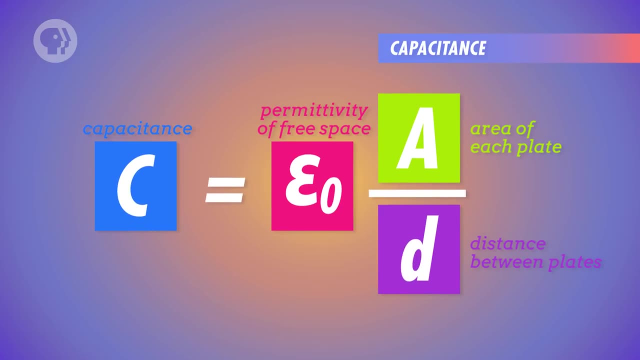 And capacitance is actually determined by the size and shape of the capacitor. One way to express capacitance is to divide the area of each plate by the distance between them and multiply that by a constant known as the permittivity of free space, denoted by epsilon-naught. Make the plates larger or move them closer together, then there's room to fit more charge, creating a stronger electric field. And once you've established the geometry of the plates, the capacitance does not change, unless you stick something between them which actually increases the capacitance. 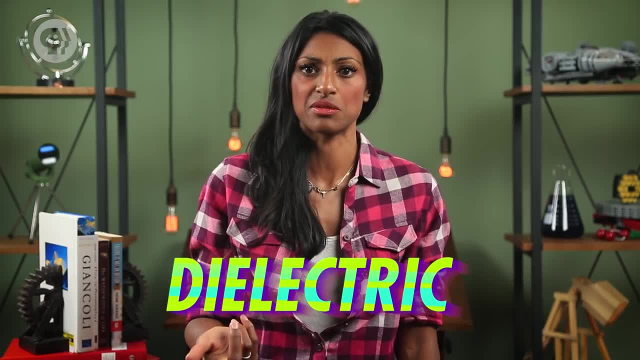 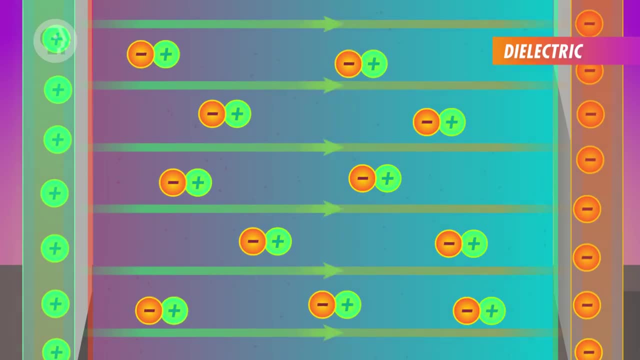 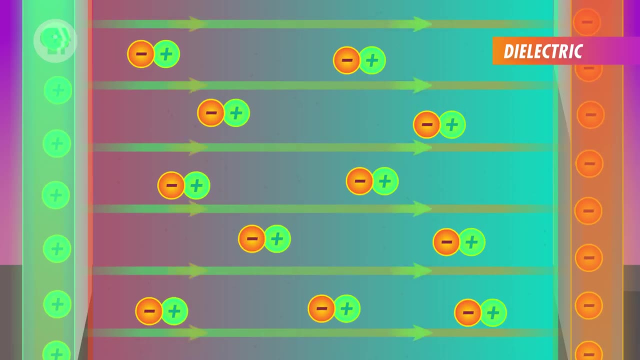 And this something is called a dielectric, Typically an insulating material like plastic or glass. A dielectric is used to increase capacitance while preventing any charge from jumping from plate to plate. Sometimes, as the plates get hotter or the voltage gets higher, some electrons naturally jump between the plates, decreasing the amount of stored charge. 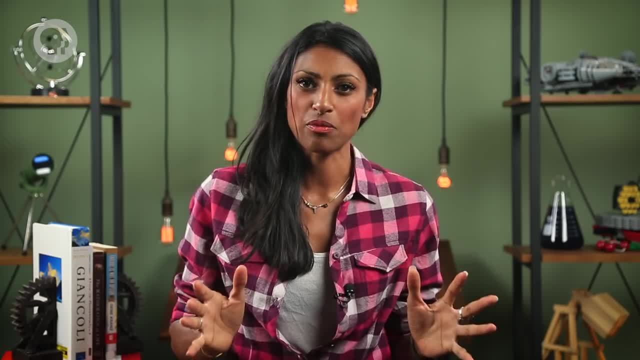 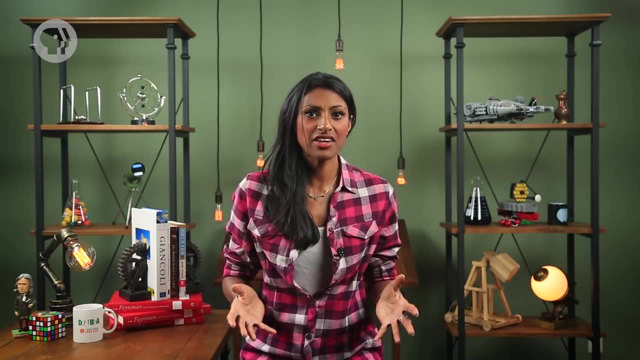 So an insulator prevents electrons from crossing the gap, And you usually want the plates to be as close together as possible without touching, since a smaller distance equals a larger capacitance. So by using a very thin dielectric the distance is decreased. 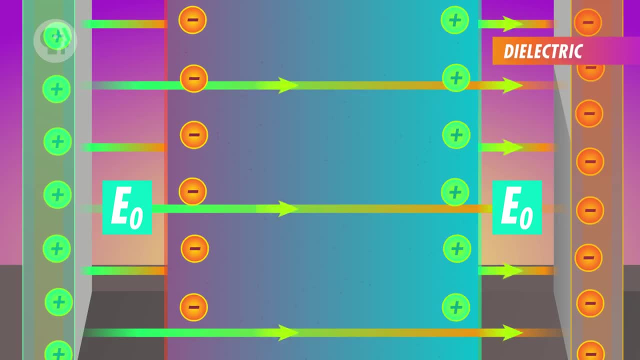 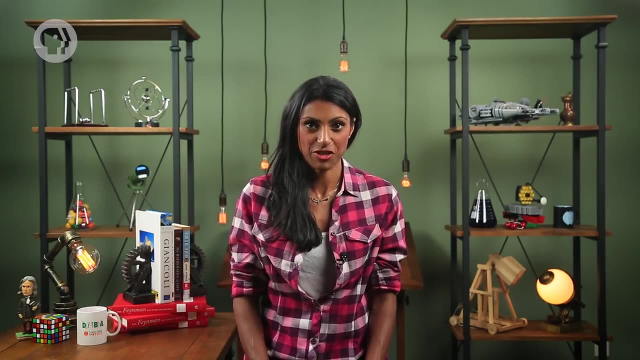 while the plates remain separate And the molecules that make up dielectrics are polar, which means one side of the molecule is slightly positive, while the other side is slightly negative, The molecules align themselves with the electric field and generate their own field in the opposite direction. 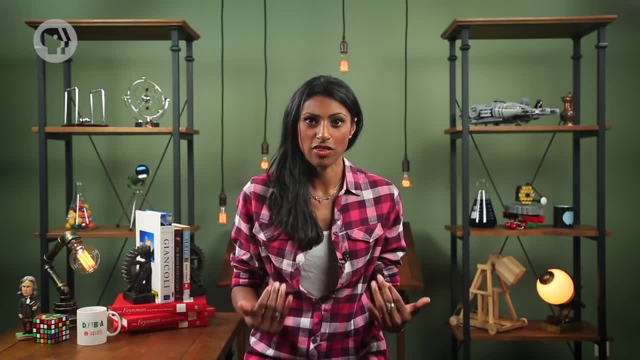 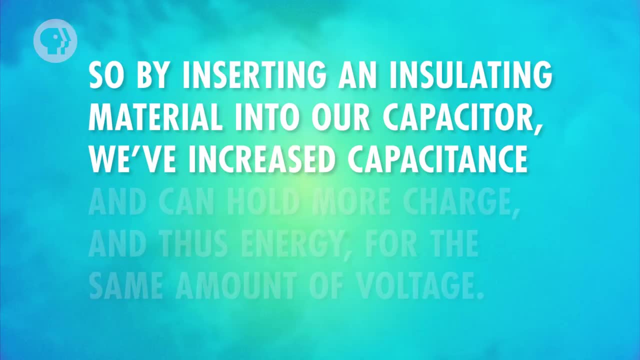 resulting in an overall weaker electric field, while the plates retain the same amount of charge. So by inserting an insulating material into our capacitor, we've increased capacitance and can hold more charge and thus energy, for the same amount of voltage. 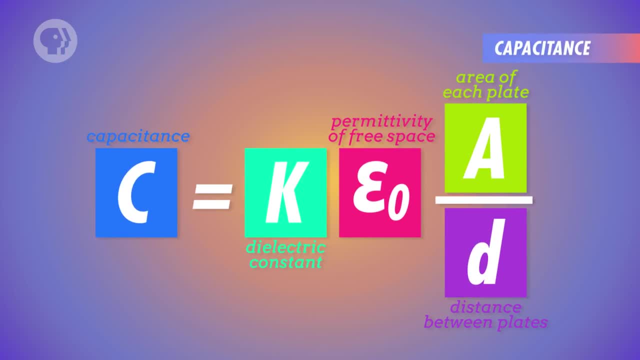 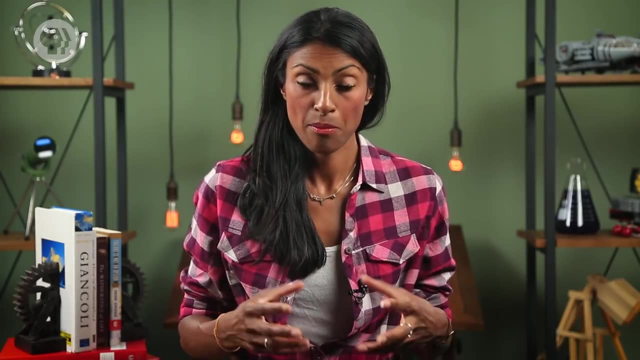 And that's why the full equation for capacitance is this. The full equation for capacitance includes a dielectric constant K, So dielectrics can help capacitors hold even more energy, and that potential energy is actually stored within the electric field between the capacitor's charged plates. 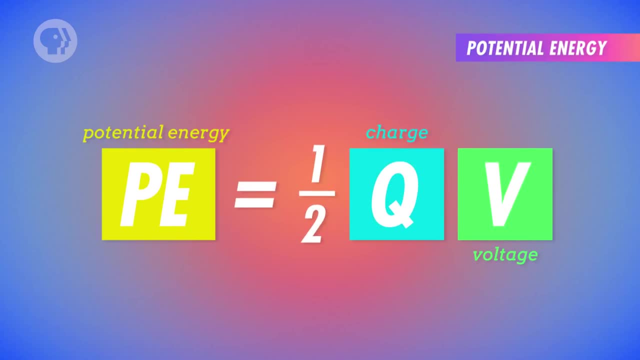 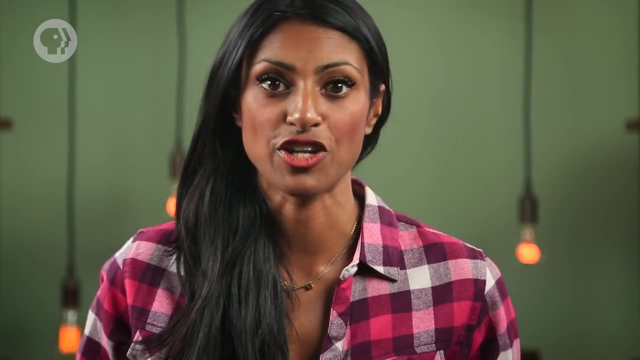 We can calculate the potential energy stored in this field by integrating the voltage over the charge in the plates, which reduces down to one-half charge times voltage. But when using a capacitor it's useful to know how much energy is stored in an electric field per unit volume. 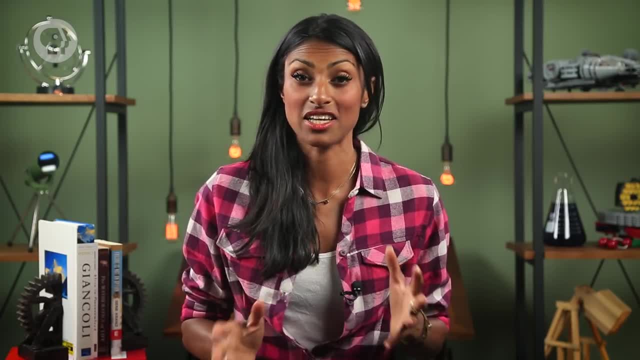 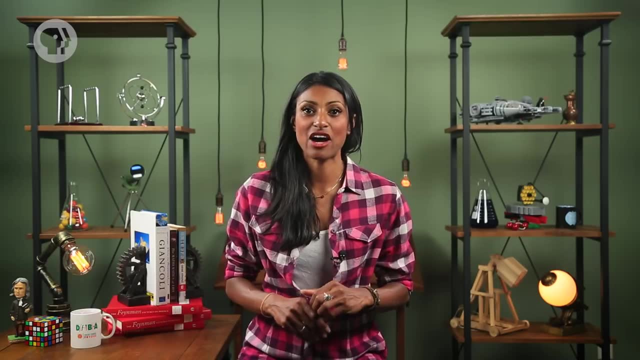 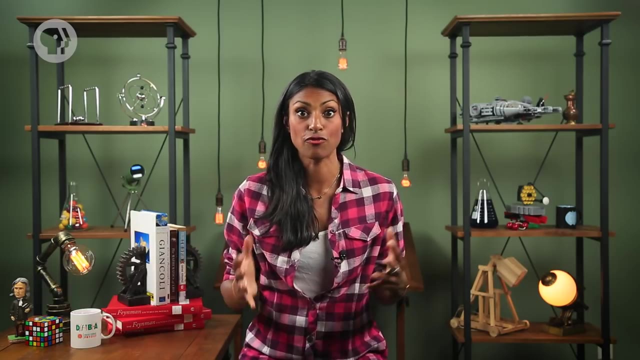 We often want to know how much energy is in a certain location, like between capacitor plates. So we use energy density, or the amount of energy stored in the electric field per unit volume, And we can calculate the energy density associated with an electric field at any point in space by dividing the potential energy by the volume between the plates. 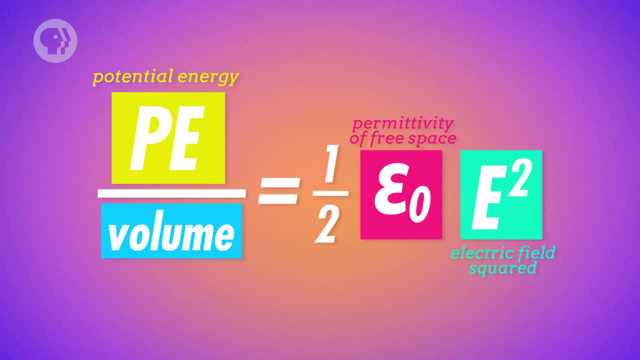 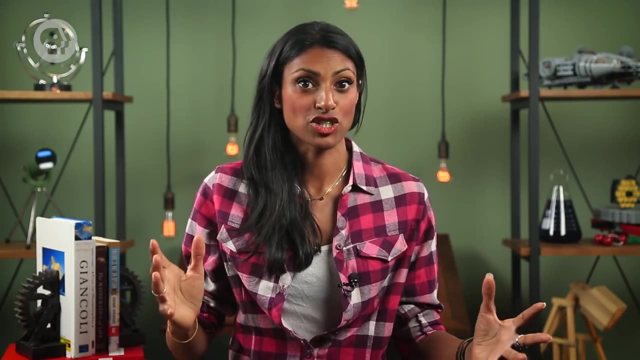 With some algebra, we find that this boils down to one-half epsilon-naught times the electric field squared, And this relation holds true for any space with an electric field. Now that we know all this, a medic can make sure those defibrillator paddles have the right capacitance. 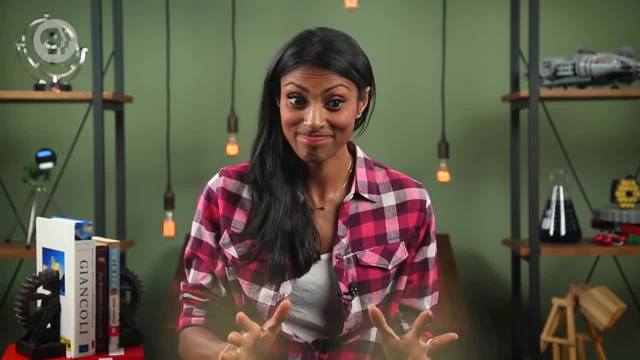 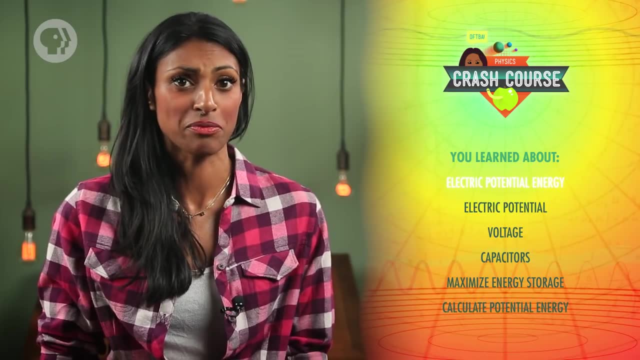 have been given enough charge to create a high voltage. and then clear Physics to the rescue. Today we learned a lot. We talked about electric potential, energy and how it differs from electric potential or voltage. We discussed how capacitors function and the factors that determine how much charge they hold. 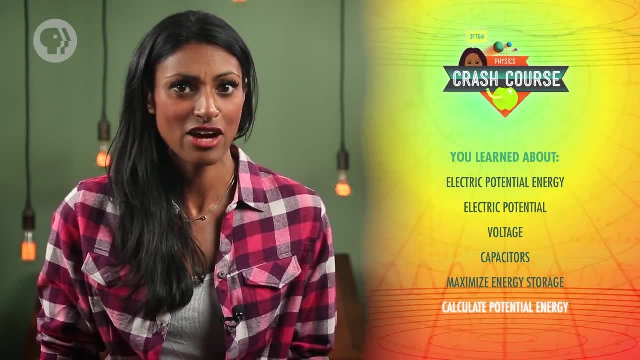 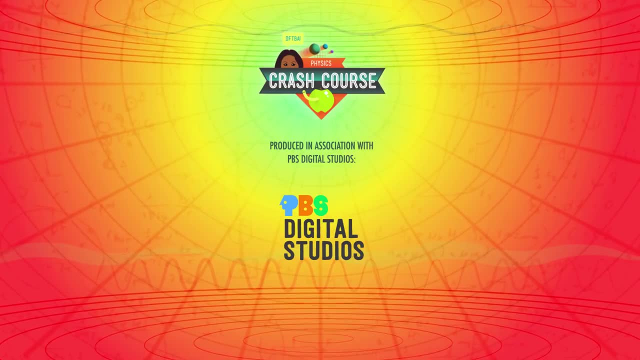 We also learned how to maximize energy storage and how to calculate the potential energy held by any capacitor. Crash Course Physics is produced in association with PBS Digital Studios. You can head over to their channel and check out a playlist of the latest episodes from shows like First Person, PBS Off Book and PBS Game Show. 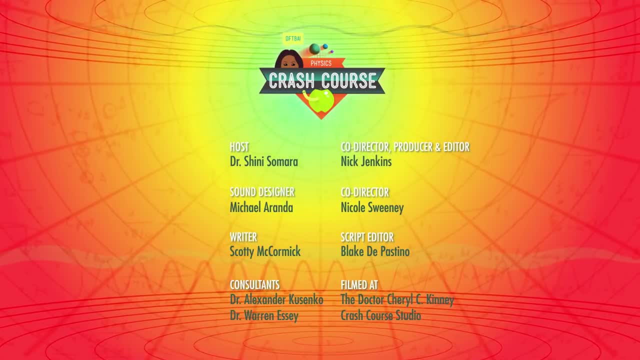 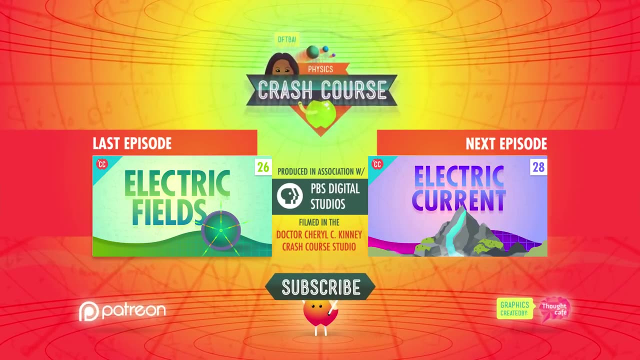 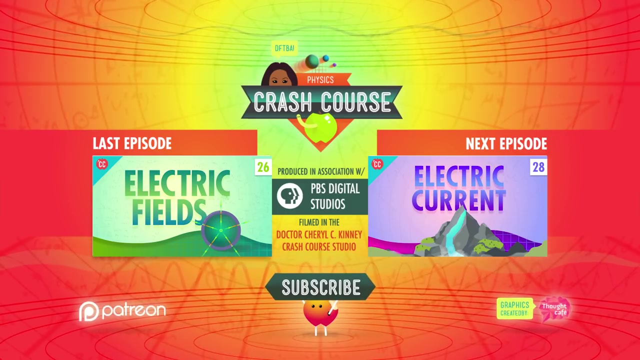 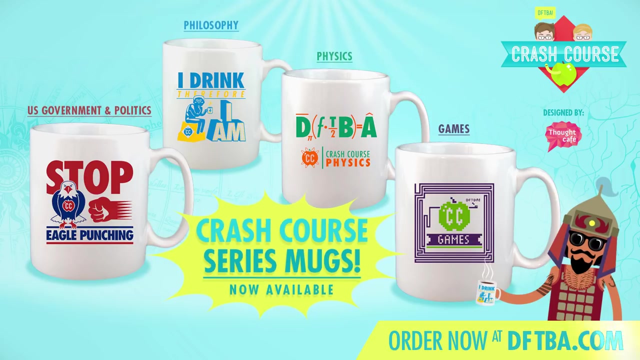 This episode of Crash Course was filmed with the Doctor, Cheryl C Kinney. Crash Course Studio, with the help of these amazing people and our equally amazing graphics team, is Thought Cafe. Thanks for watching. We'll see you next time. Thanks for watching.